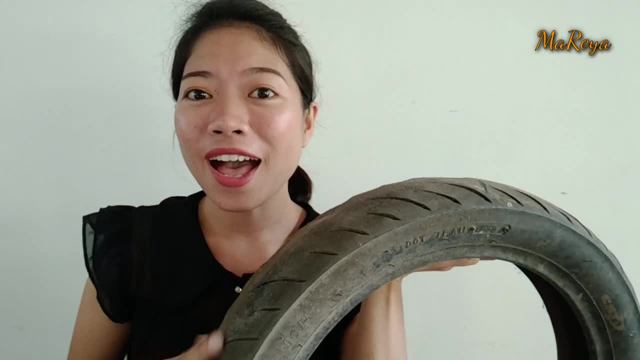 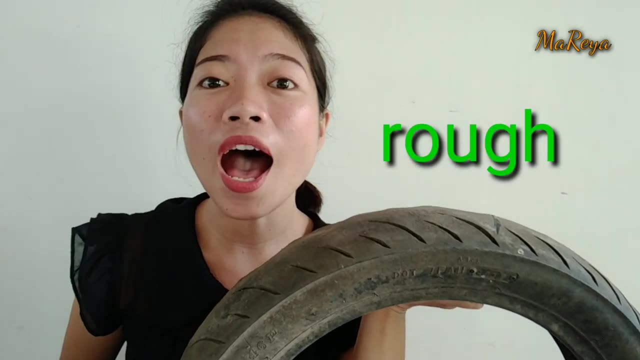 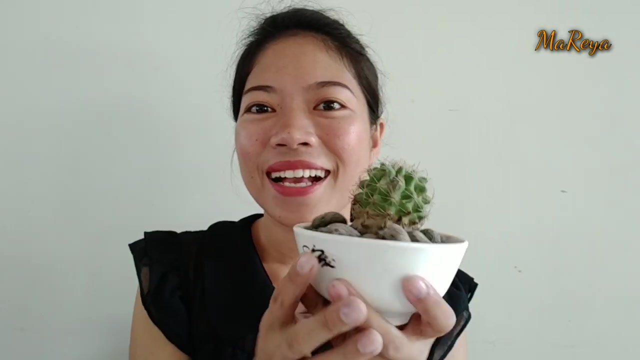 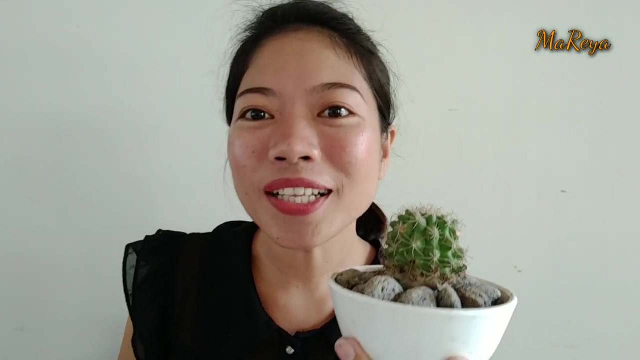 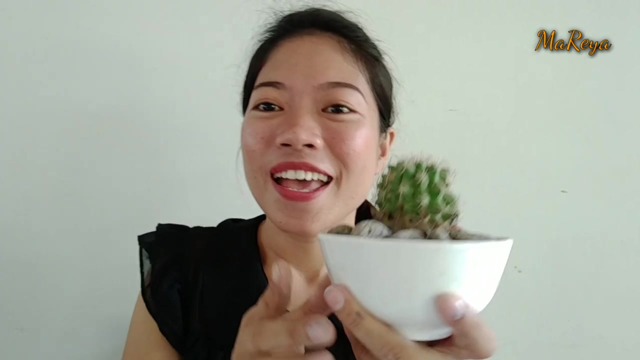 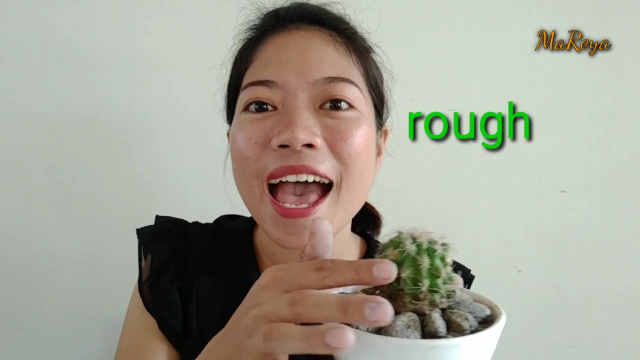 Rough or smooth. Touch, touch, touch. A wheel has a rough surface. This wheel has a rough surface. Cactus- Touch, touch, touch. What can you feel? Smooth or rough, Smooth or rough? Rough Cactus has a rough surface. Cactus has a rough surface. 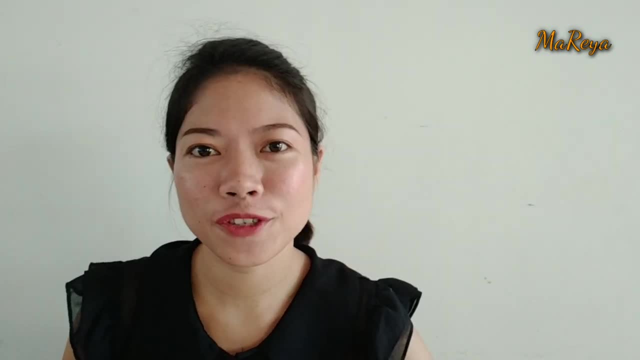 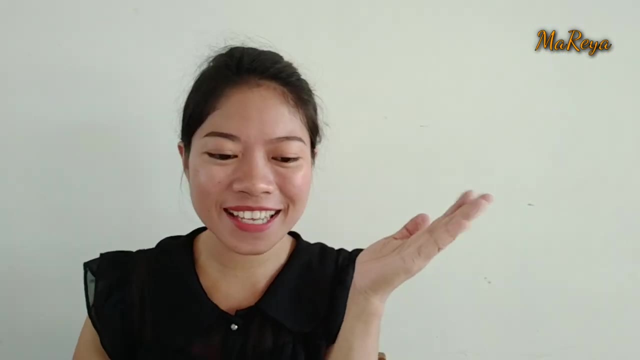 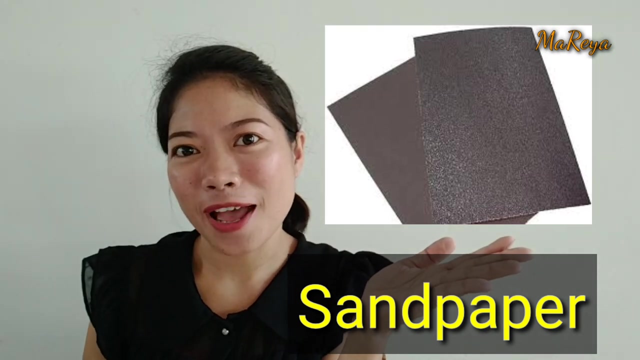 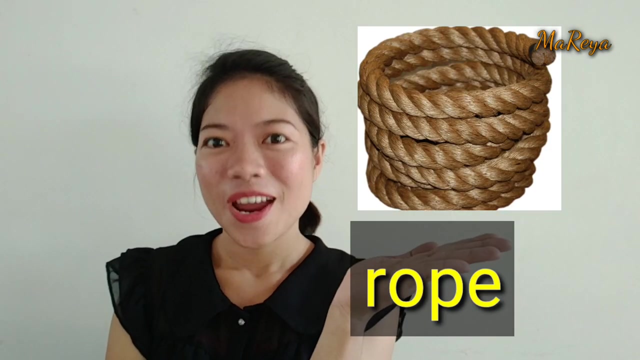 There are many things that has a rough surface, Just like Dorian. Dorian has a rough surface right, And also sandpaper. Sandpaper also has a rough surface. Coconut, It has a rough surface. A rope Rope has a rough surface. Try to touch it and you will know. 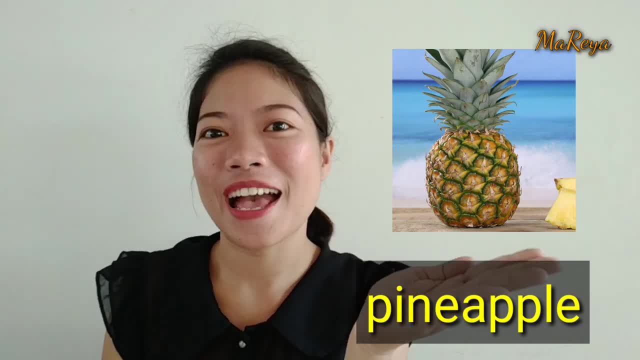 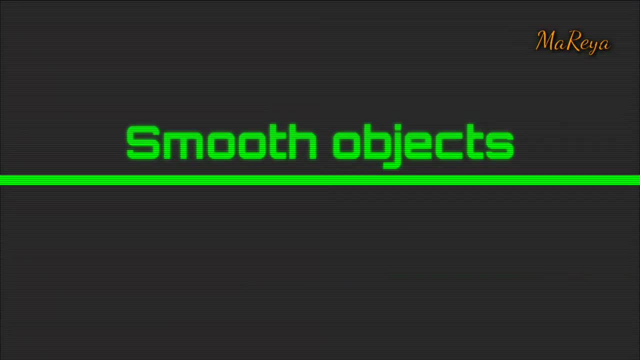 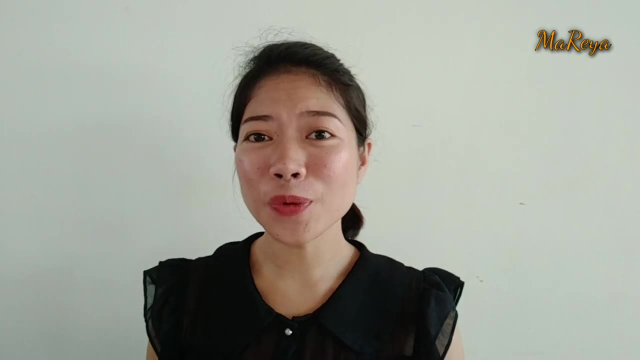 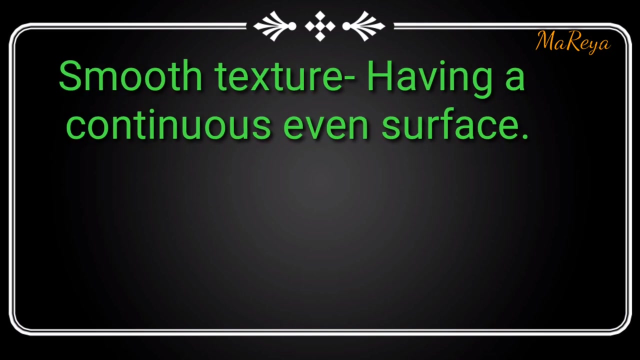 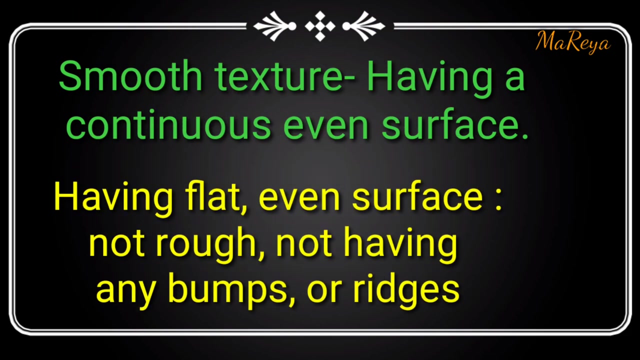 Pineapple. Pineapple has a rough surface, Corals- They have rough surface. So now let's discuss what is a smooth or smooth objects. Smooth surfaces: Smooth texture, Having continuous, even surface, Having flat, even surface, Not rough, not having any bumps or ridges. 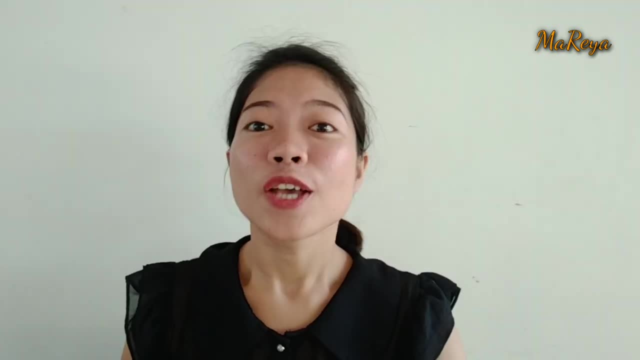 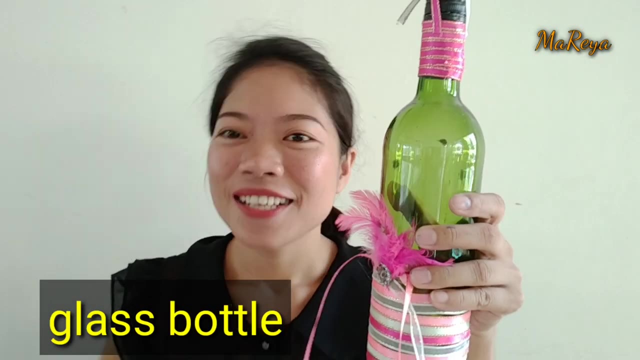 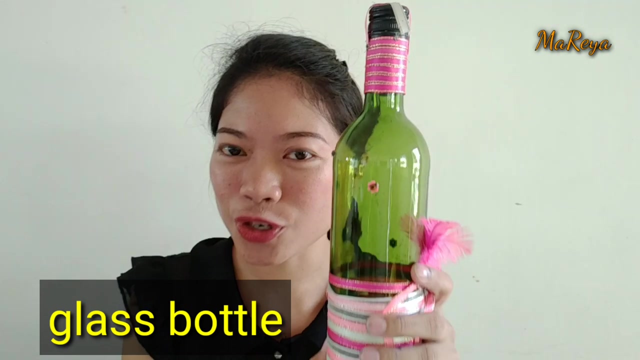 I will show you things that has smooth surface. I will show you things that has smooth surface. I will show you things that has smooth surface. Ok, now A bottle. Use your hand, Touch, touch touch. What is the texture? Smooth or rough? Touch, touch, touch.